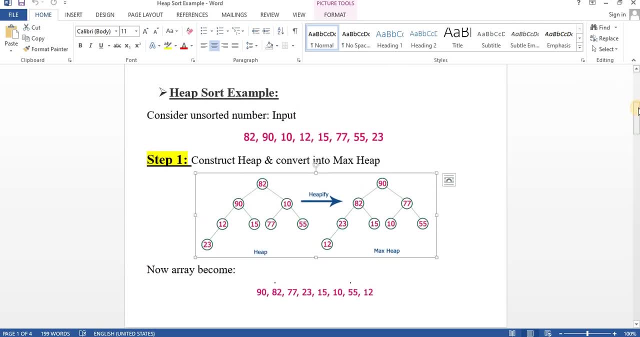 first just review the example. If you know the example of hip sort, then only you should understand the C++ program. Okay, So hip sort is one kind of data structure. They sort the particular data. If you pass input as a unsorted array, then they convert this input into the sorted form, either in maximum hip, or it means ascending order, or in minimum hip means descending order. Clear, This is the aim of hip sort algorithm. So this is the one of 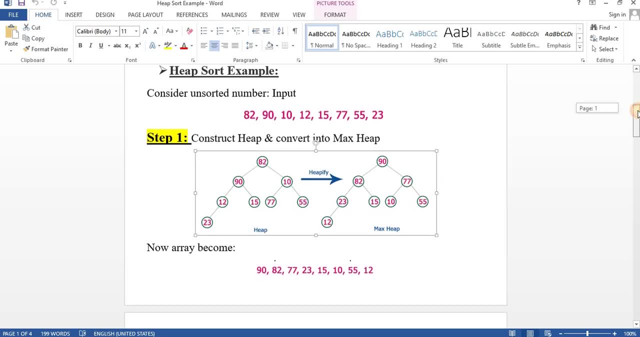 the oldest hip sort algorithm for sorting purpose. Now just review this example first, See here: your input is unsorted array. See here 82,, 90,, 10 up to 23.. This is your unsorted array. Now you need to convert this unsorted array into the sorted form by using hip sort. The first step is you need to convert this array into the binary tree format- See here: this is a unsorted array- and convert it into the binary tree format. Your first node 82, which consider 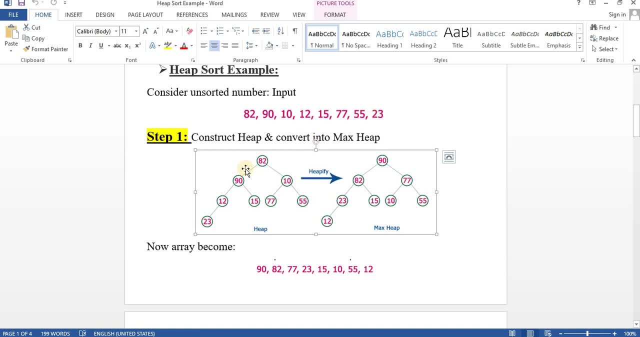 as a root node and after that all the remaining elements have added from left to right in binary tree, like 90,, 10,, 12,, 15,, 77,, 55,, 23. in this way, This is the first step: Convert unsorted array into the binary tree. Second step is you need to apply hippify function on this binary tree. Hippify function is a logic of hip sort. The logic of hip sort is compare every left subtree element with the root node. After that, right. 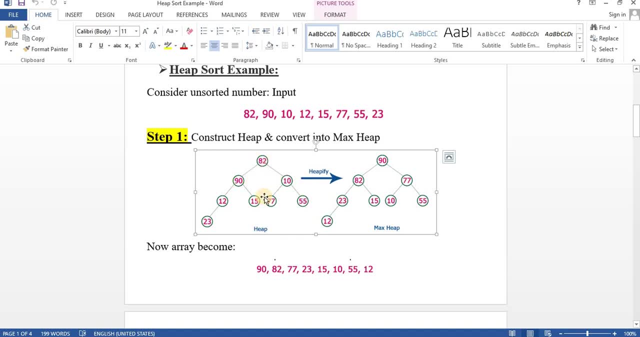 subtree element with the root node Means every root node is the largest and their child node is the lowest element. Okay, In this way, See here: Here: 90 first compare with 82. 90 is greater than 82. Swap it or interchange it, So 90 become root node, 82 become child node in this way. After that, suppose 82 is here, 82 compare with 12.. 82 is larger. Take as it is Now. 12 is compared with 23.. So 23 is largest. Swap it or interchange it. 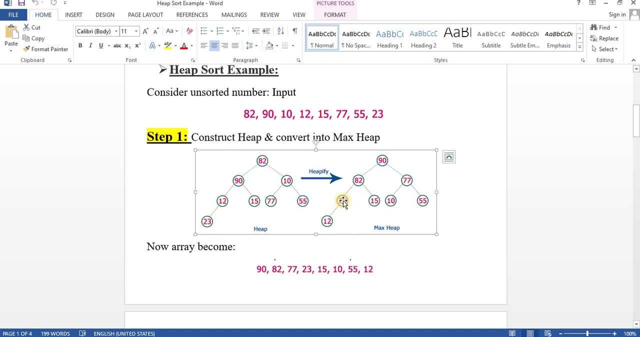 So 23 goes to here and 12 become child node in this way. Okay, Similarly, here, in this right subtree, here 10 is compared with 82.. 82 is largest. Take as it is Now. 77 is compared with 10.. 77 is the largest, So 77 become a root node and 10 become a child node, and similarly 55. So 55 is smaller than 77. Now, after applying hippify, this binary tree will be formed. Now, see here, focused here, This binary tree is 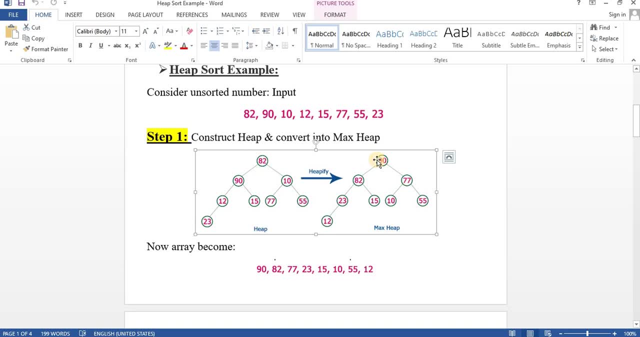 is the maximum hip binary tree. every root node is the largest: 90 is larger than 82 and 77, 82 is larger than 23 and 15, 23 larger than 12 here, 77 larger than 10 and 15. correct, now this maximum hip is again converted into the array: see here. now 90 is a root node and remaining 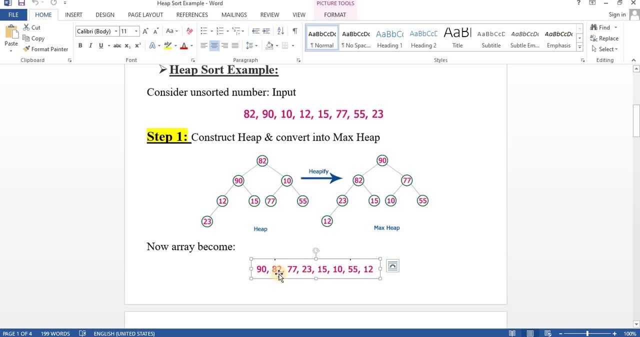 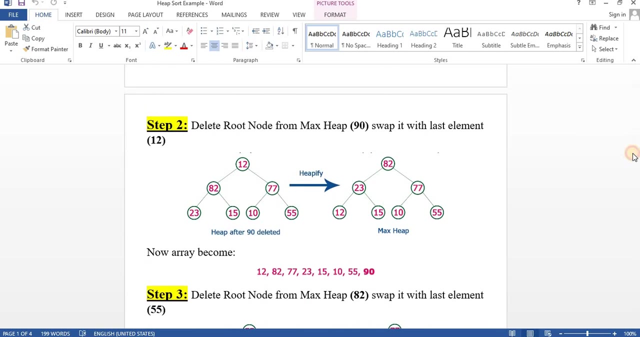 tree as it is. so print this maximum hip into the array format 82, 77 up to the 12. now see here: this is the sorted array. no, now goes to next step, that is step 2. okay, the logic of next step 2 is in binary, in hip sort. see here, which is a root node in maximum hip 90. 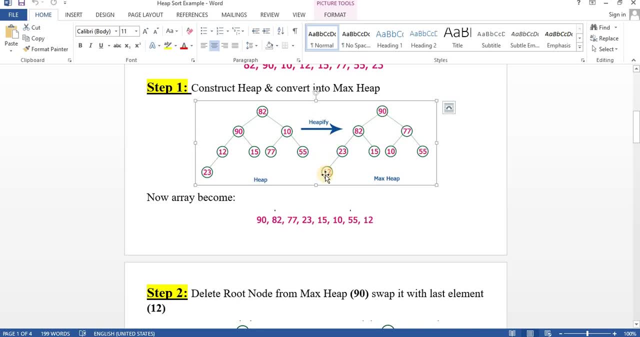 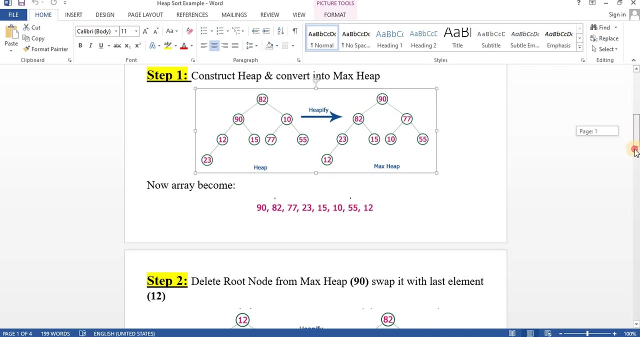 so delete those root node. replace with the last node in the tree, which is the last node, 12. so 12 placed at the 90 and 90 become deleted. now this deleted element stored into the one another array. this is your sorted array. okay, so this 90 will be deleted. now 90 stored into this array. this is your sorted array. 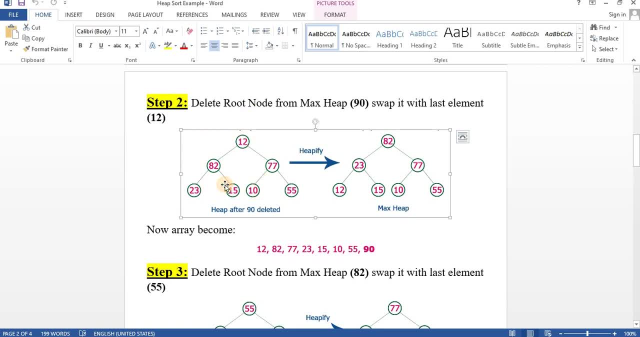 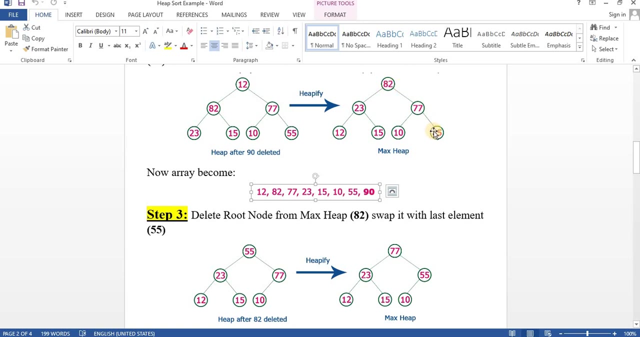 okay, now again, after deleting 90, this binary tree will generate right now. apply hippify on this binary tree, hip sort logic same. this array will be generated now. this is the unsorted array again. perform. delete root node, that is 82. replace with last node, that is 55. so 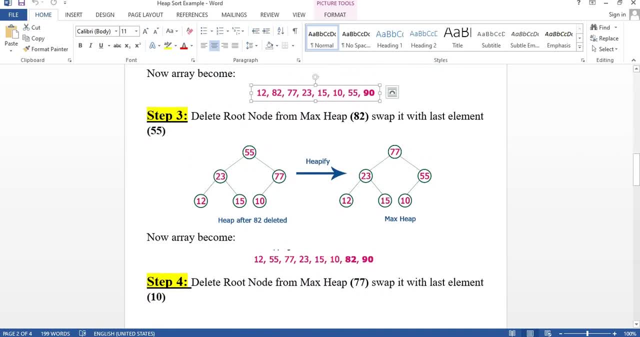 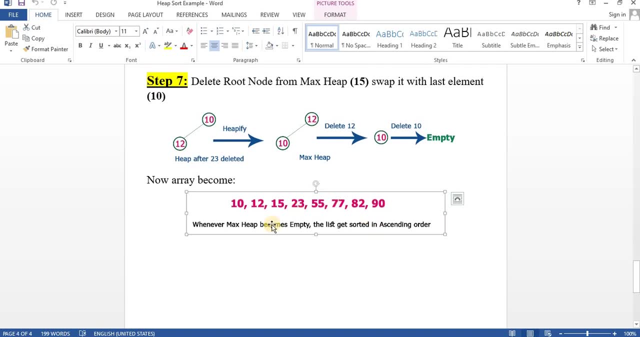 this deleted element stored into the sorted array. so in this way, you need to perform these steps on each and every binary tree and at the end this array will be generate right. first, 90 will be deleted, after that 82, after that 77. in this way: 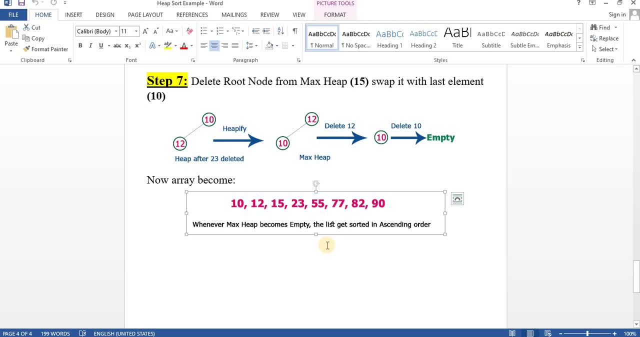 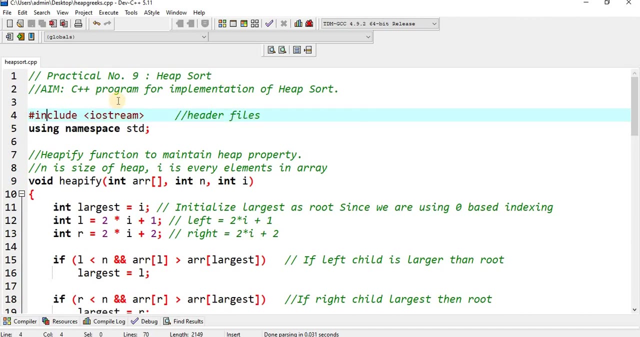 see here: this is a sorted array, so in this way hip sort algorithm will work. clear. now we will discuss this example in C++ program format. okay, now see here. this is a C++ implementation of hip sort. first your header files. we need to import header files because it stored all. 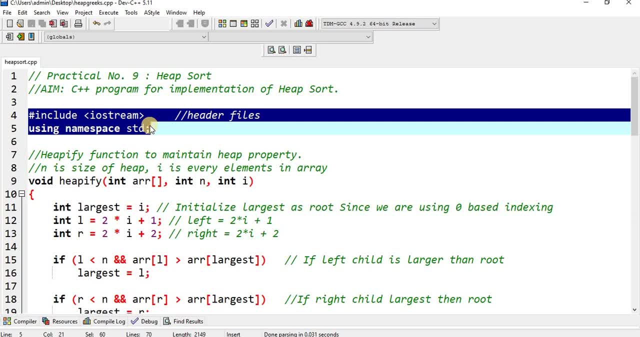 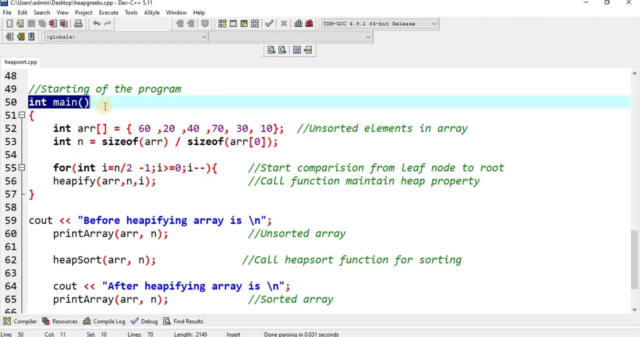 the built-in functions and variables like see out, seen, and all the functions have so stored here. so first input input output stream dot edge this header file clear. so after a importing header file your program always start with the main function. okay, this is your integer main function. now in main function here I have declared one array you can see. 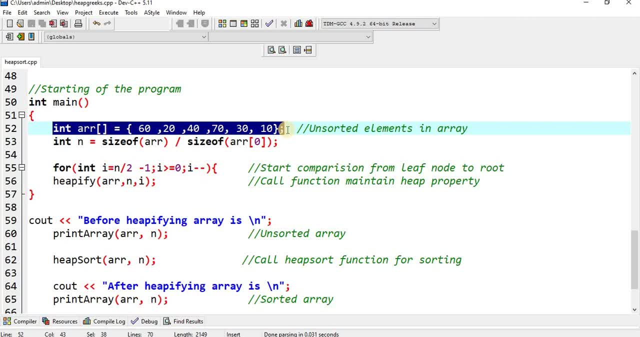 you can take also input as a runtime, like when after executing the program there will be a message: enter the elements. and you can enter unsorted elements. so you can perform that way also. but here I am taking one array. the array name is ARRR. now in this array there are total. 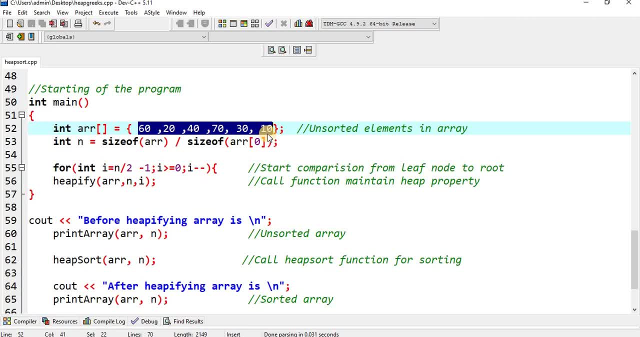 six element: 60, 20, 40, 70, 30 and 10. this is the unsorted elements. okay, now you need to convert this unsorted array into the sorted array format by using hip sort. okay, this is a logic. now, here, the next step is you need to perform size of array divided by size of array of. 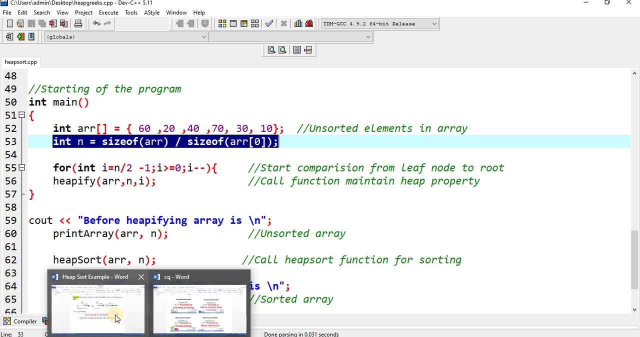 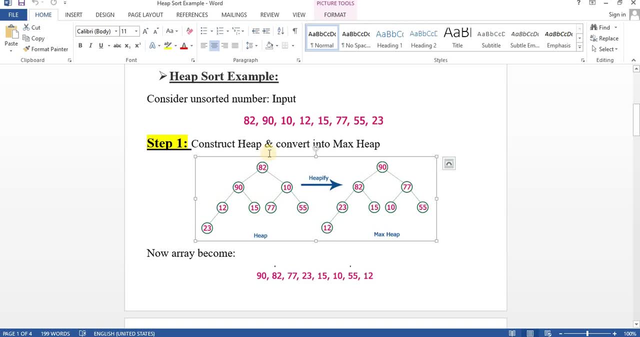 0 means: see here the meaning of this line is in our example. you need to convert this array into the binary tree format. right, the first node become a root node. remaining half elements goes to left side and half element goes to right side. right means you need to. 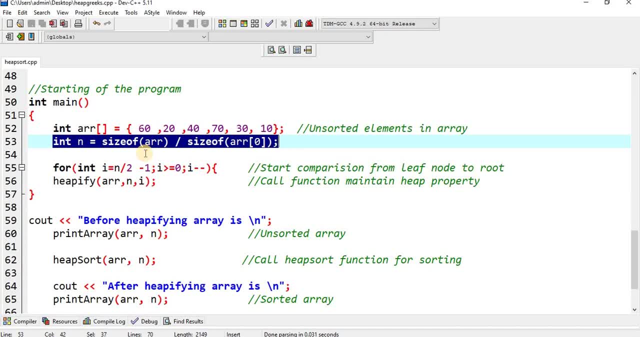 divide the array into the format. that's why this formula is applied here on the total number of elements. clear now you need to divide those elements. means start comparison from the left node to root I. and divided by two means divide array into the two format. okay means there are total eight elements. so first element: consider as a root node remaining. 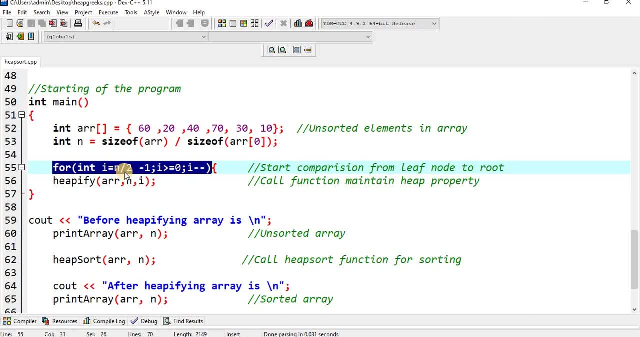 seven elements. so seven element divided into the two parts left sub tree and right sub tree. clear, that's why we used here I and divided by two minus one. so this is a formula now up to I. greater than equal to 0 means you need to apply this logic up to the 0th. 0 means root. 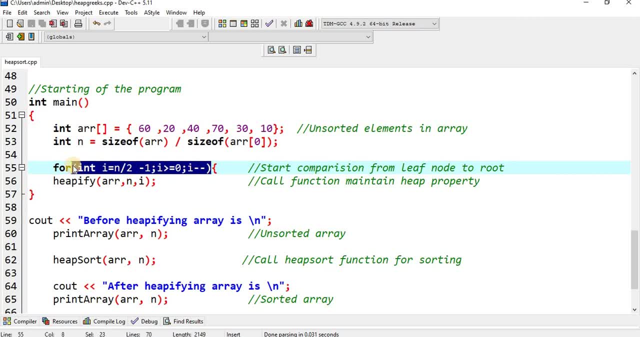 node clear and I minus minus. in this way you need to generate a binary tree as per your unsorted array. so after generating binary tree you need to call hippify function. so hippify function pass three parameters. array means you are a total array. this unsorted 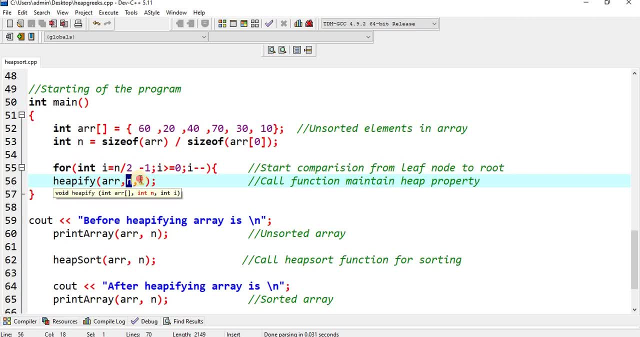 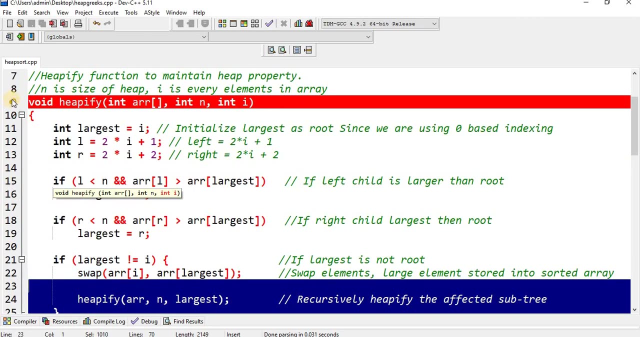 array and means total number of elements in array and I means the root node. okay, I consider as a root node. so these three parameters pass to the hippify function. now they call hippify function. see, we declared hippify function afterward the main function. okay, now just. 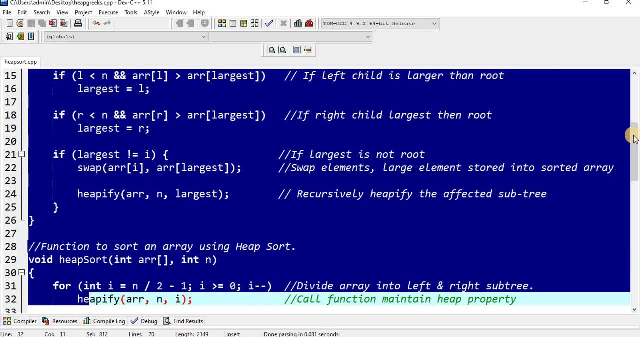 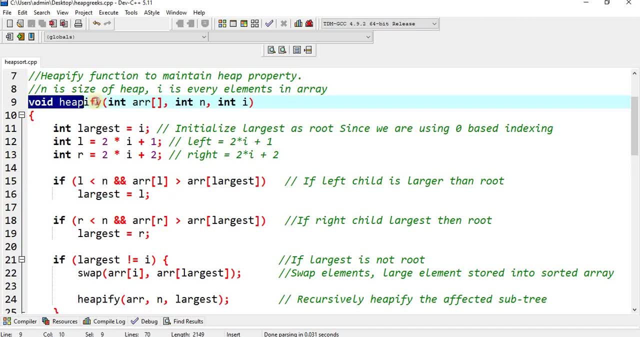 focus here. this is a main logic of hip sort algorithm. you need to just understand the logic, so you need to perform practicals carefully. so the first is hippify function. see here void hippify. they pass three parameters: your array, total number of array and the root node. now 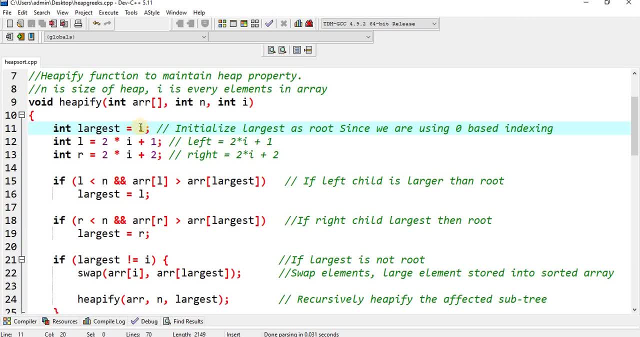 integer I. largest. equal to I means your I is equal to largest. largest means your root node. okay, whatever the your root node is stored into the largest variable. clear now. next, so there is a integer L and integer R. L means left, R means right. 2 into I plus 1. this element. 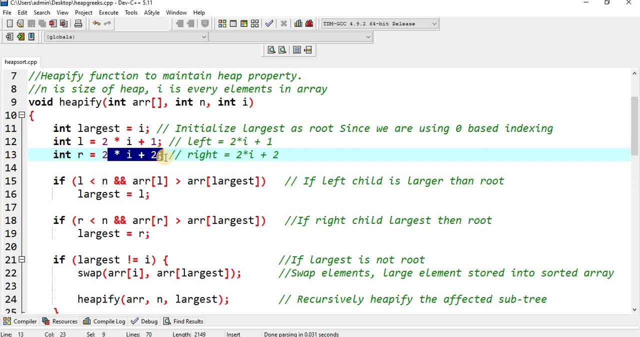 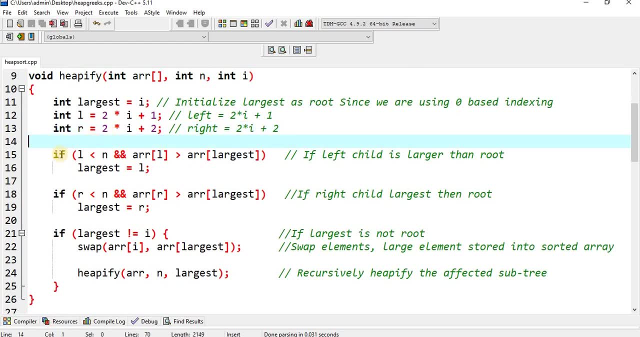 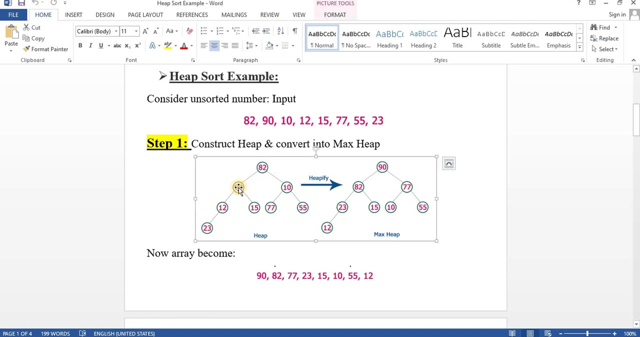 goes to left side as a left subtree and 2 into I plus 2, this element goes to right subtree. okay, as per the formula. Now, see here. the next step is: see here, as per our example, the next step is: after generating binary tree, you need to compare the elements first. you need to compare 90 with 82. 90 is 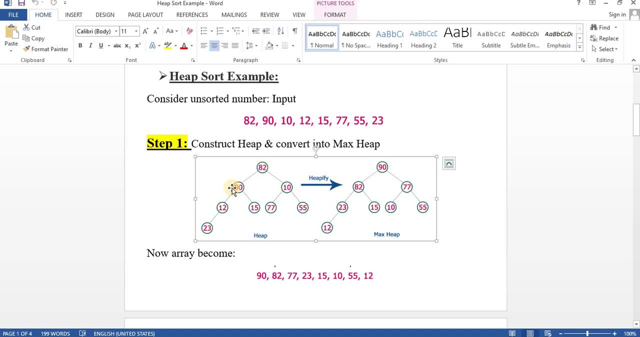 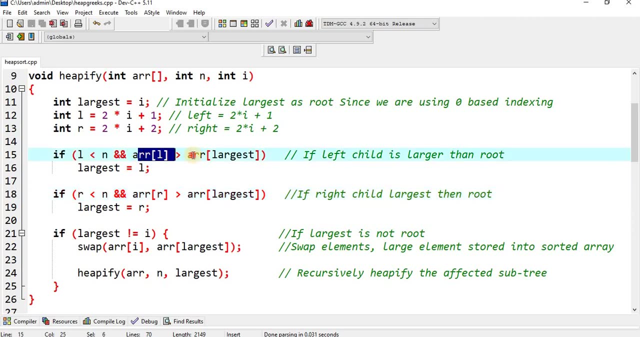 greater than 82. so 90 move to root node, 82 move to child node in this way. so this logic apply here. see here you need to compare left subtree value with the root node. array of L means left subtree first value And L means left subtree first value. 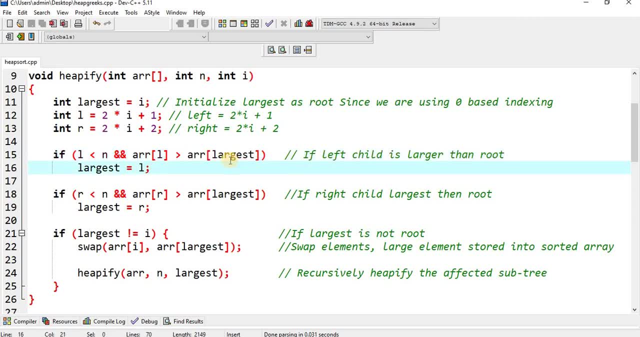 Array of largest means root node. okay, if left child is larger than root node, then you need to perform the swapping operation. okay, you need to swap those element: root node become a child node and child node become a root node in this way clear. similarly, on the right: 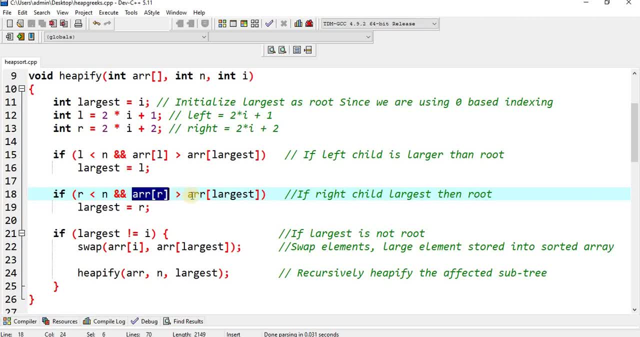 side, right side, compare right subtree value with root node and if right, child root node value, child value is greater. so again, perform the swapping operation clear. So this is a logic: left subtree comparison, after that right subtree comparison. okay means whatever the value of present they perform. the swapping operation is here clear. now again: 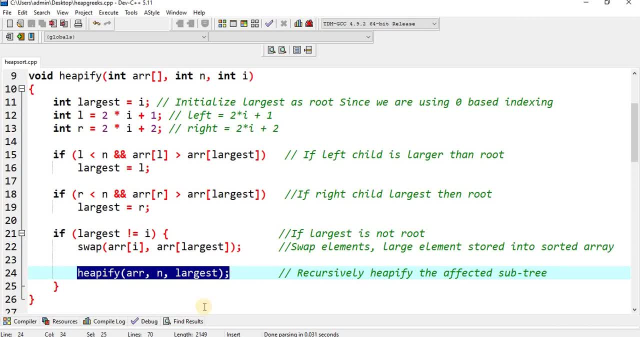 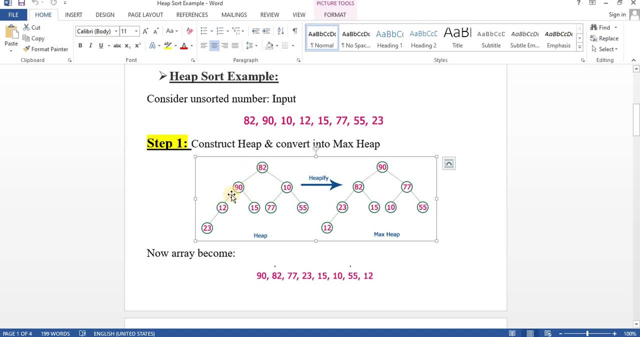 they call hippify function means recursively. they perform the comparison clear. see here: first: 90, compare with 82. 90 is greater than 82. perform swapping. again 12, compare with 90, a smaller, which take as it is. so you need to perform recursively each and every time. 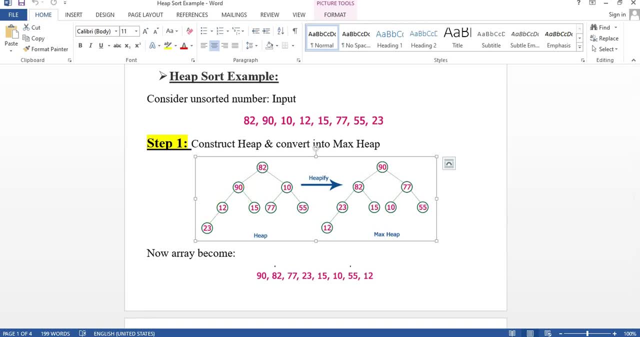 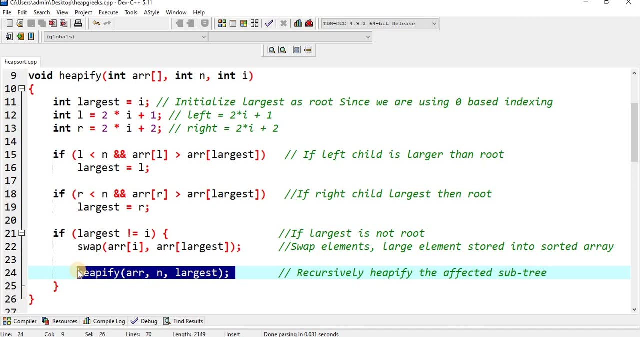 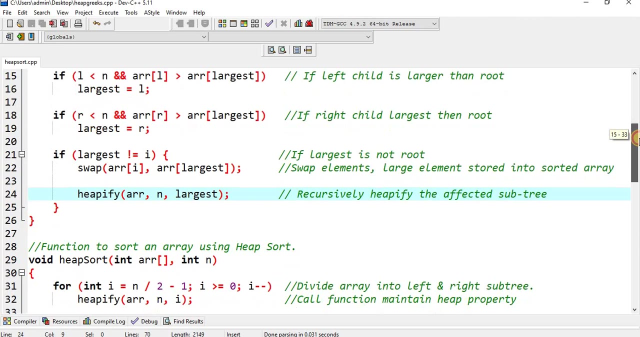 every node is compared with the another node clear. so that's why they call hippify function up to the all the elements have sorted format. okay means step one, two, step six or seven. this all the way they call the hippify function: recursively clear. this is a logic of the program. 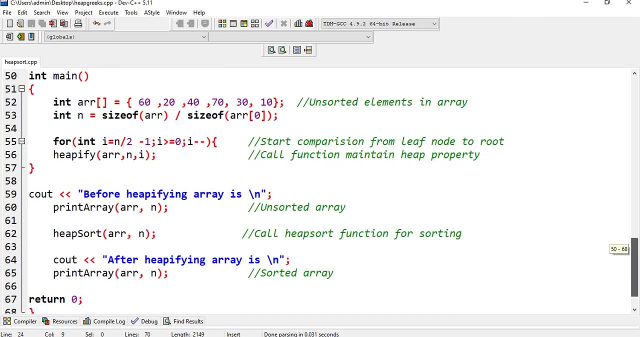 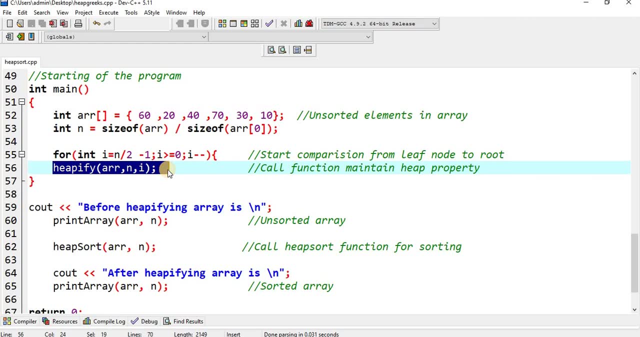 after that, see here. so in main, function the array generate a binary tree and they call hippify function. So hippify function Generate a hippify or maximum hip binary tree, as per the logic. now, after that, after performing this thing, the next is they: when you execute a program, they apply, they show the one message. 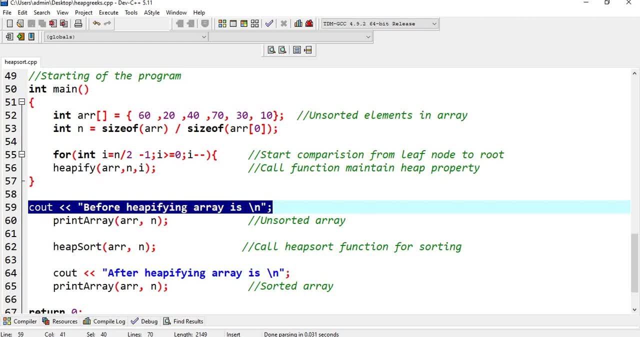 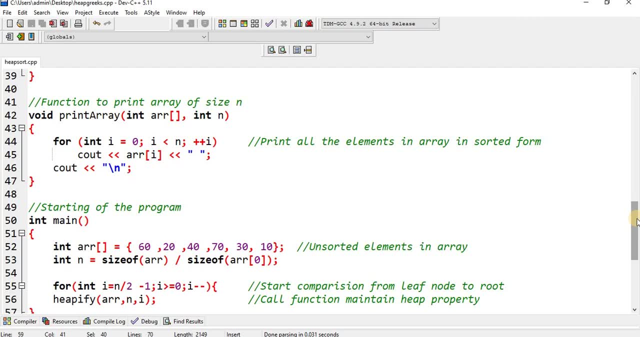 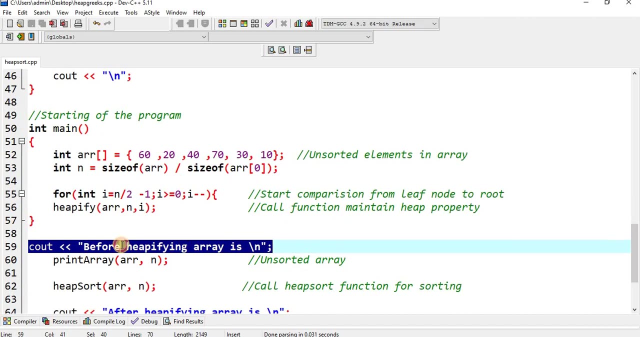 like before hippifying array, print array, array of n, so print array function we declared here okay. so means when you execute a program they will show you the unsorted array first and after that they show you the sorted array. In this two message: Okay means before apply, before applying hippify array, and after hippifying array. in this way: 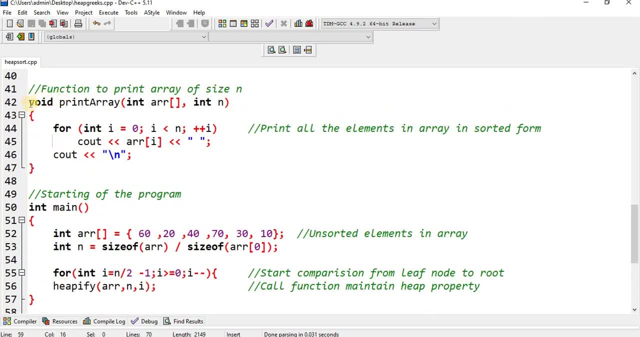 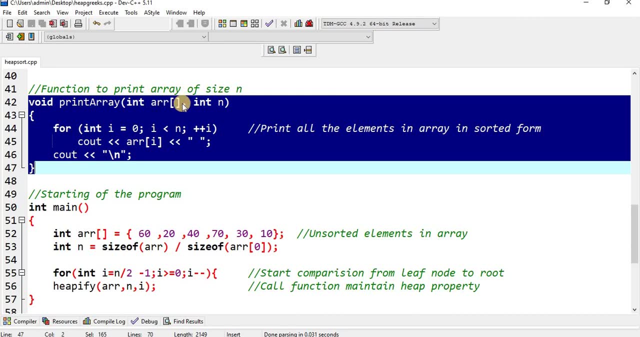 so they call a print array function. so here I'm taking one again: print array function. see here: void print array. they pass two parameters: array, your unsorted array, and total number of elements in array. so they check the elements from i is equal to zero to i less than equal. 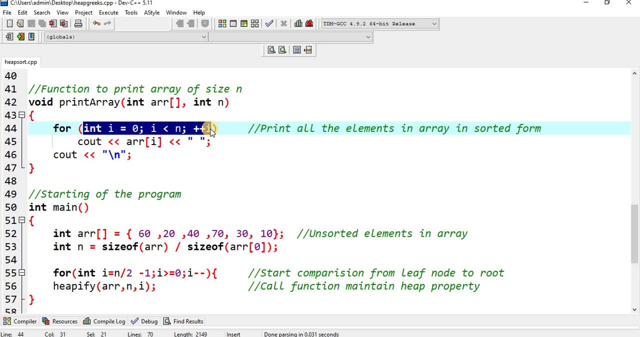 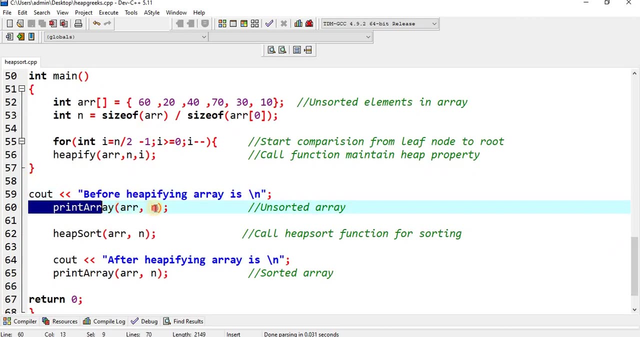 to n. i plus plus means from. there are total six elements in array from zero to five. So one by one all the arrays have printed and this array have stored into this array of. i clear, so see here before hippifying arrays: print array array of n means they print this. 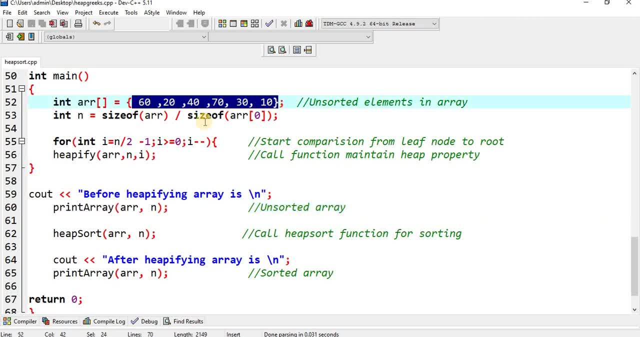 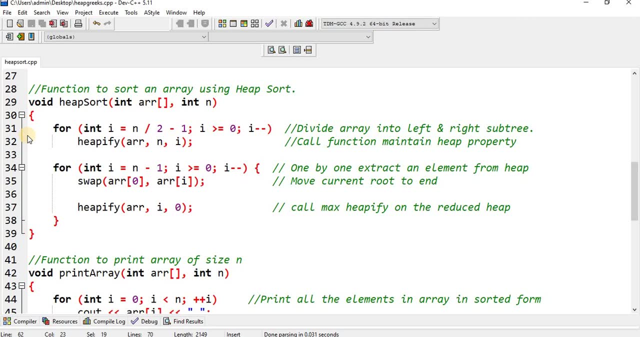 unsorted array as it is as your input they print as it is. now they call hip sort function. okay, so hip sort function means, see here, there are total three function: hippify, hip sort and print array. okay, so, see here, this is a hip sort function. 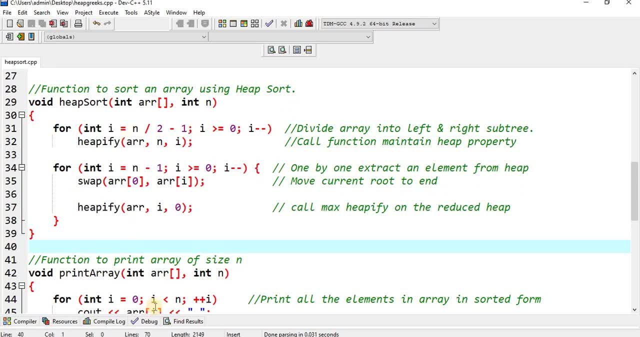 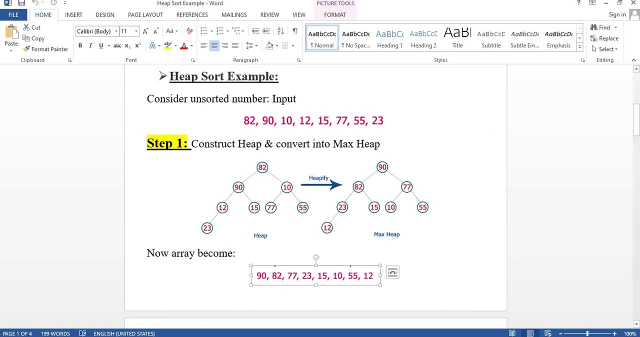 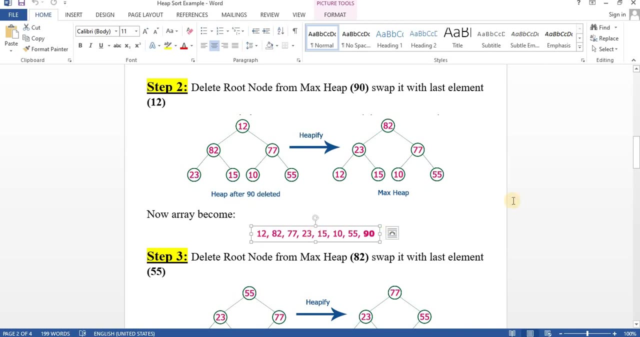 Basically They just sort the elements. okay, see here, see here in this example: every time this new array will be generate, right, whatever the deleted element is. first you delete the ninety element, so ninety element, this array will be generate. after that, eighty two will be deleted, this array will be generate. so for generating this array purpose, you need to. 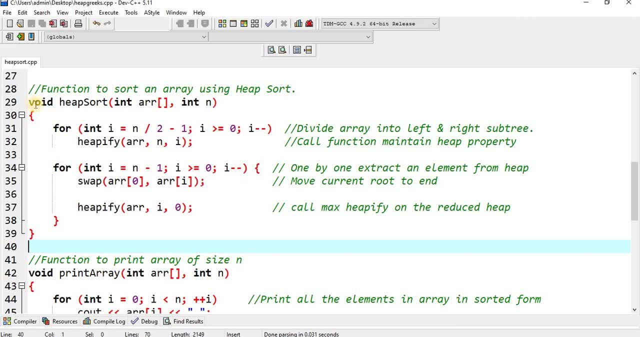 use hip sort function. okay, so see here this is a hip sort function. First they divide the array from left and right subtree, right, and divided by two minus one, i greater than equal to zero, i minus minus. this is a for loop for dividing array from left subtree and right subtree. then they call hippify function. hippify function, convert. 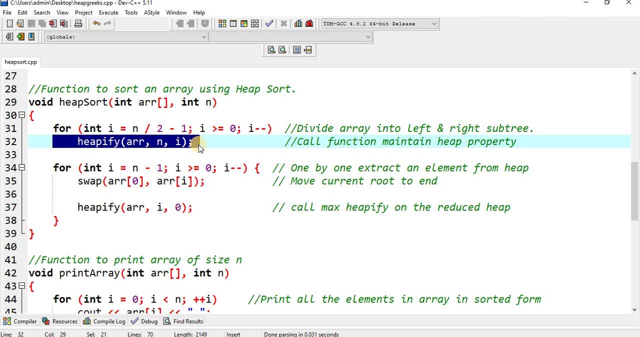 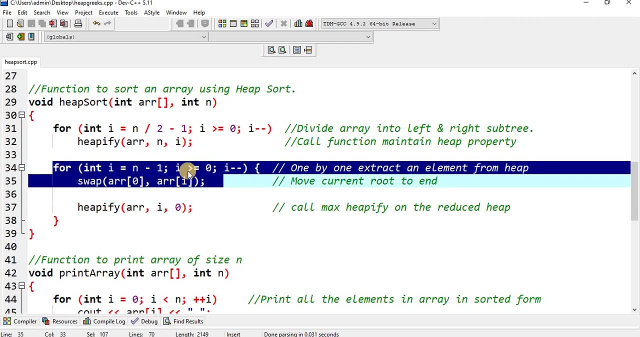 your binary tree into the maximum hip binary tree right, and after that. if array is not sorted, then they extract the element. okay, They Take the first root node. see, here, i is equal to n minus one means the first element, the first root node, that is the greatest one. so they extract those element and in this way, 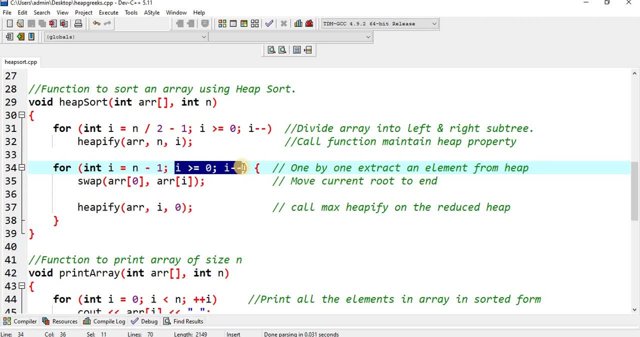 every binary tree. i minus minus will be perform right. so they extract one by one element from the hip tree and they print those element into this array. okay, this is a next array. there is two array: one array and one array of zero means from zero to end. they print this. 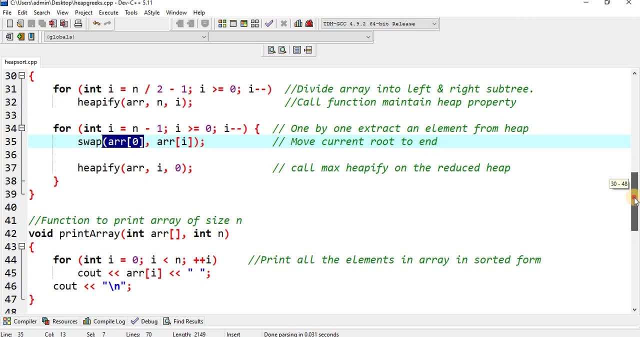 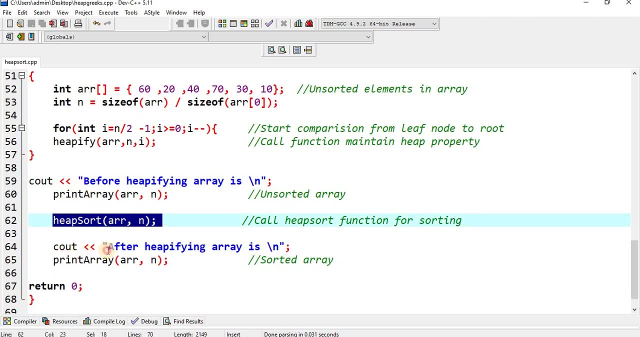 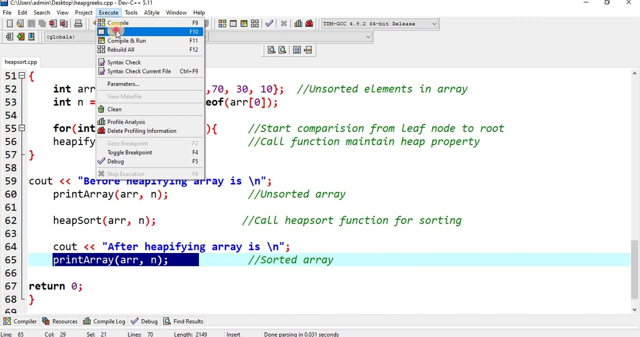 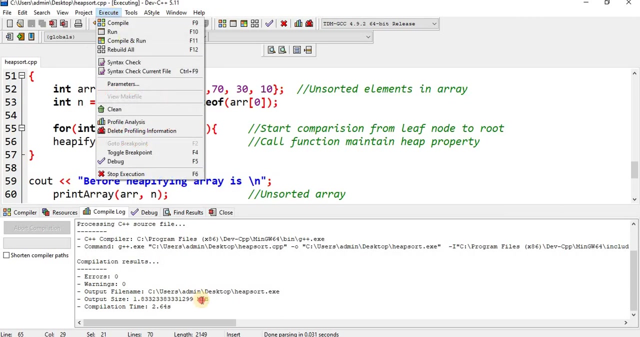 array. here i have mentioned the command for each and every line. so after that, after hip sorting, the again give the message: after hippifying array is, and after sorted array it can be printed. so just execute this program once. first i compiling this program. okay, wait a minute.